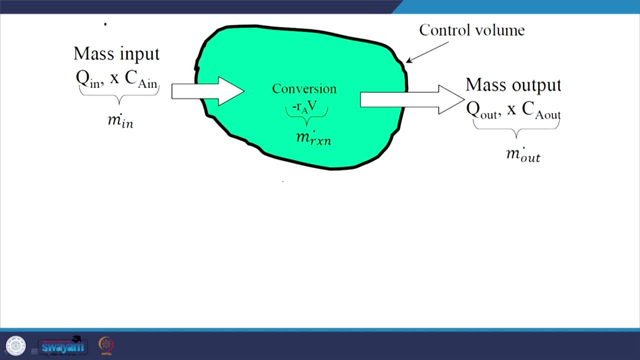 Here we have the control volume and what do we have looks like. if this is my wastewater treatment plants reactor, I have mass coming in due to flow Q in and the concentration of the compound in that input flow, and similarly flow out and the compound going out along with that flow. 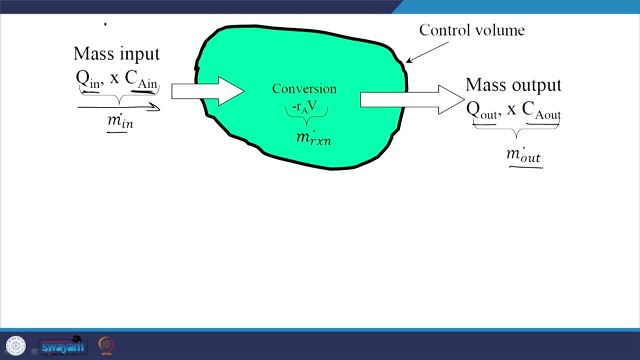 So mass coming in and mass going out and also looks like the compound is being converted due to reaction and that is due to this particular reaction here. rate of that particular loss of that compound. Why am I saying loss? Because we have a negative out here. So to put it. 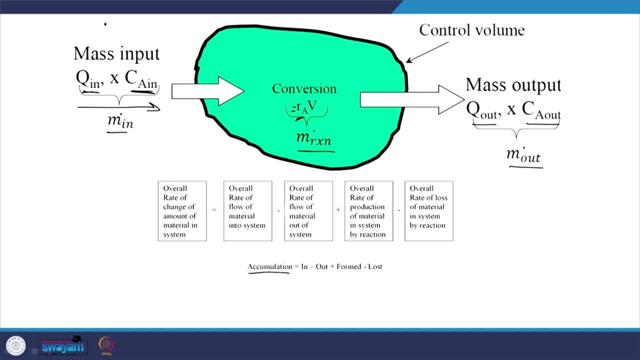 the general terms. so we have accumulation, we have mass coming in, mass going out, we have the compound being formed due to reaction, compound being lost due to the reaction. So if I put this in terms of the variables that I am going to use, so I have d Vc by 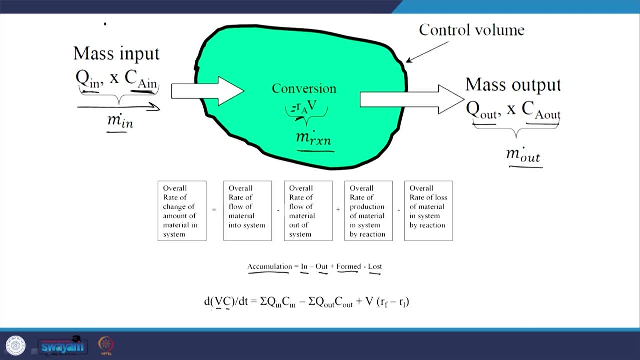 dt V into C is nothing but mass, as in V is volume and concentration is mass per volume, And so if these two will cancel out, I am left with mass. so it is nothing but change in mass per time within that control volume. 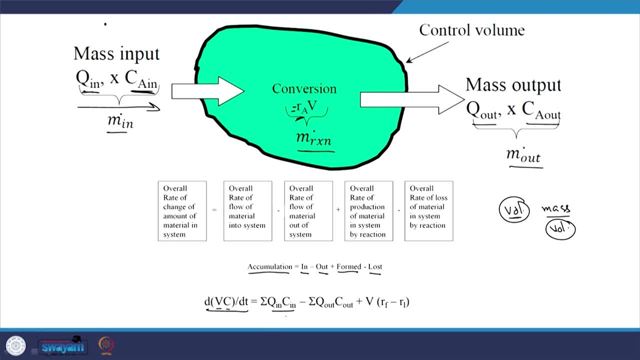 Summation of all the mass coming in via the flow or due to advection- here Q in, C in, that is something that we looked at- And all the flow That is leading to loss of the mass or mass output. So mass in and mass out. 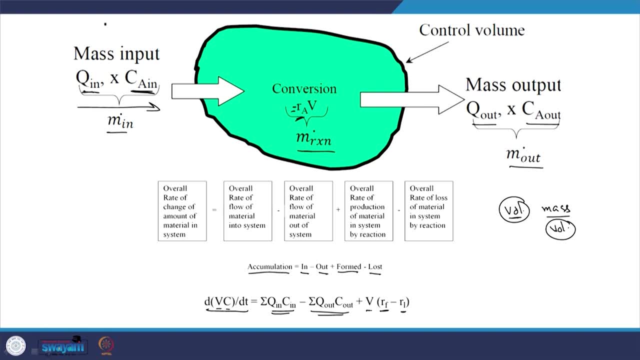 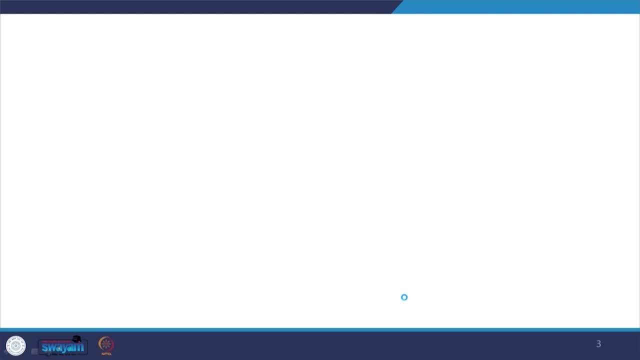 And then the compound being formed or lost and we multiply by volume so that the units stay the same here. So that is what we have out here. Let us see how I can transform that particular equation. What do we have? We had d, Vc by dt- change in mass per time within that control volume is equal to the. 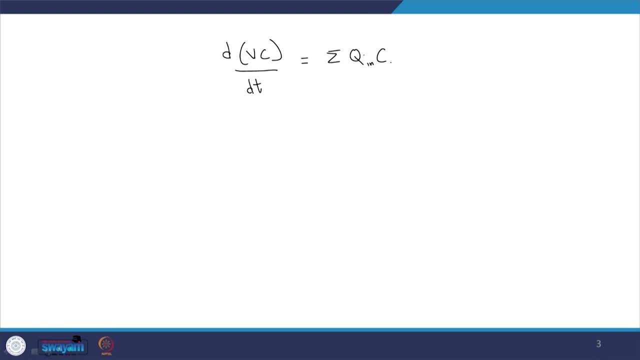 summation of Q in And C in, or mass coming in minus mass leaving via this advection or leaving the relevant reactor. let us see, need not say advection out here, Q out into C, out plus volume into rate of formation of the compound, minus rate of loss. 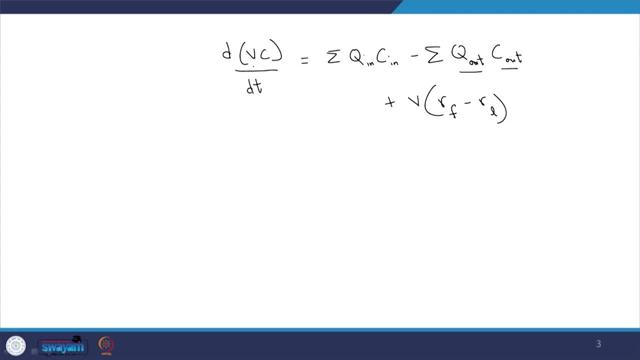 of the compound Right First this term. typically the volume of your reactor is constant, so V does not change with time. So V, dc by dt Is equal to all these terms. let us see. So that is what we have out here. 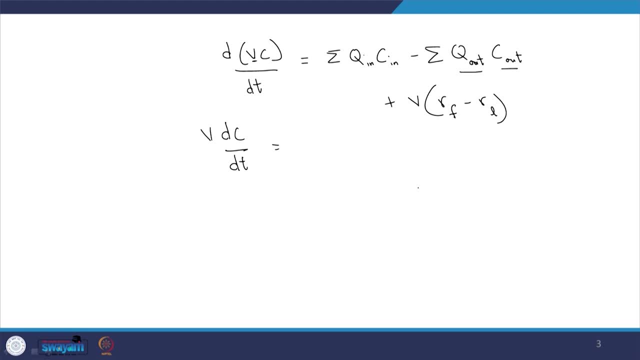 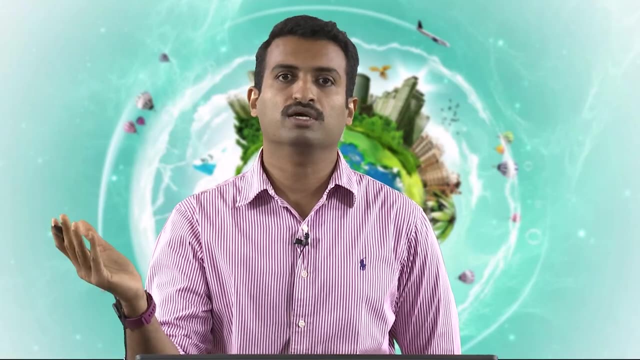 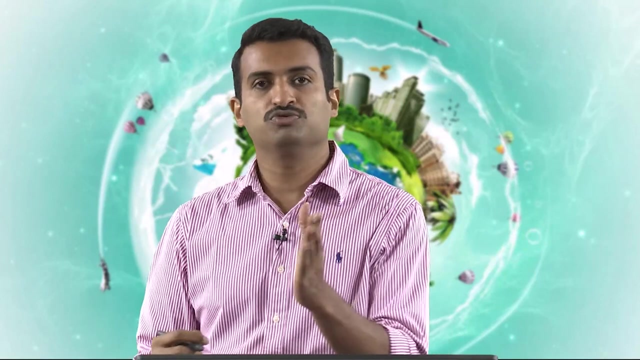 And we can transform this according to the type of reactor that we have. For example, this room now is closed, the door is closed, all the windows are closed. So if I release some compound here right now, at time is equal to 0 and want to observe. 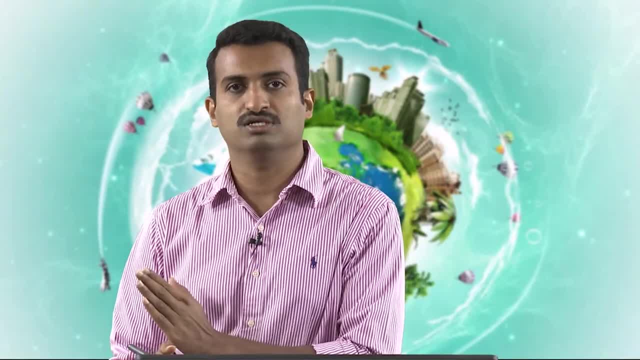 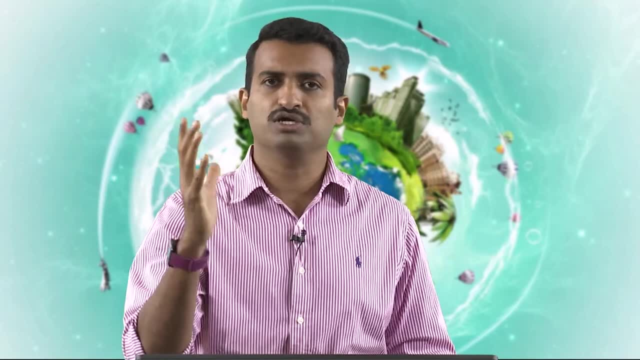 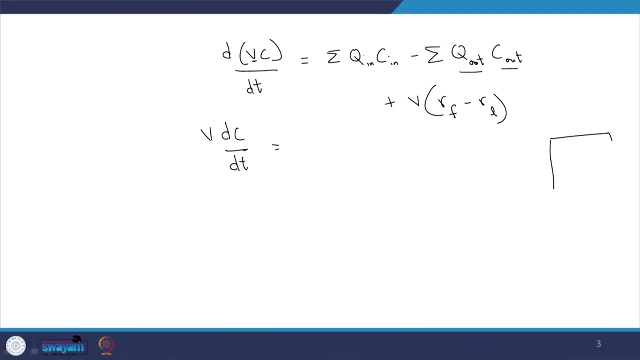 the changes in this particular reactor at different times. let us see, Right Reactor is my room. let us see, And let us say, to get the same concentration throughout the reactor, I keep the fans turned on. let us see. That means that I am having something like this, which is a closed system: a closed system. 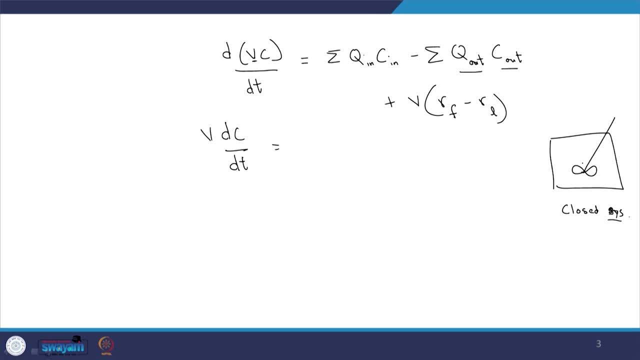 closed system and then it is continuously mixed so that the concentration within the particular reactor is assumed to be constant. let us see, But Note that because there is no flow coming in or no flow going out, What is it now? We do not have this mass term. 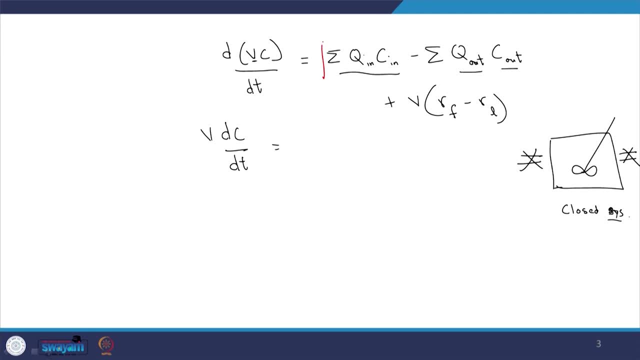 This mass term is not going to be applicable in this particular example. we are talking about the room out here. So there is no mass coming in. mass in minus, mass out is 0 and let us say we have equal to plus. So this is equal to rate of formation minus rate of loss of the compound. 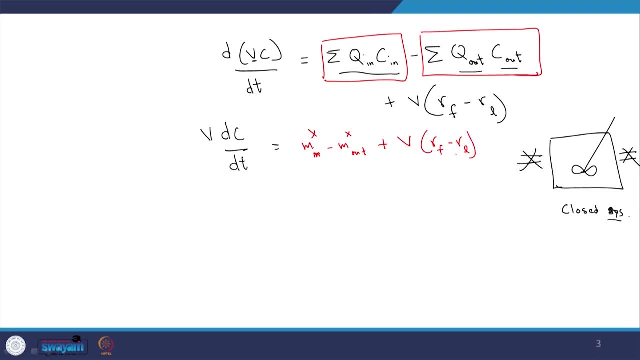 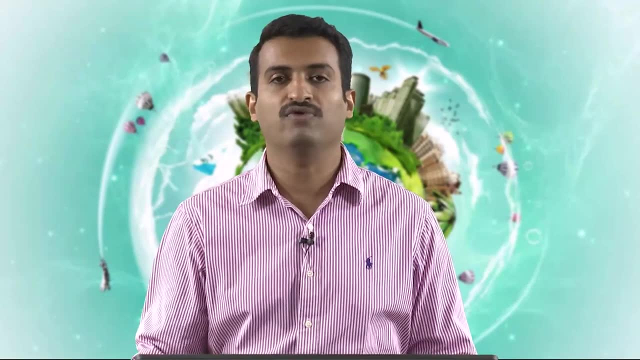 And the example I was trying to give was: let us say, I opened up this bottle and I released a particular toxin or hazardous chemical into this room and I left. the fans turned on And the person outside the room wants to know after how many minutes or hours is it safe? 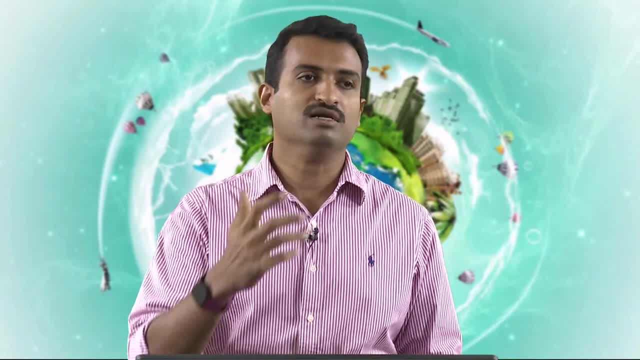 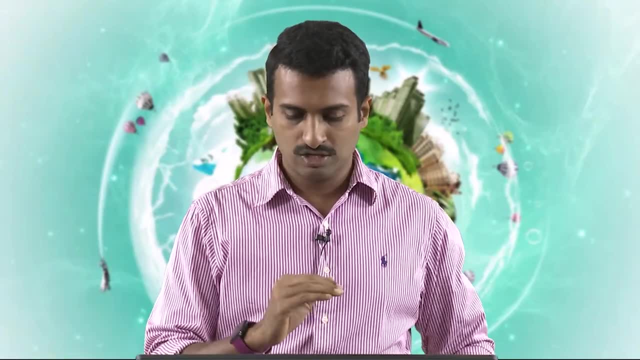 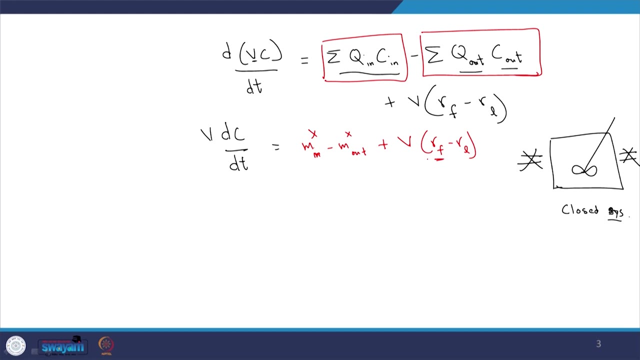 to come into this particular room, assuming that the compound will react with, let us say, oxygen in the atmosphere And, you know, Be transformed into harmless byproducts. So there is no formation of the compound, there is only one time: release. We do not need to look at that because there is no mass coming extraneously from the system. 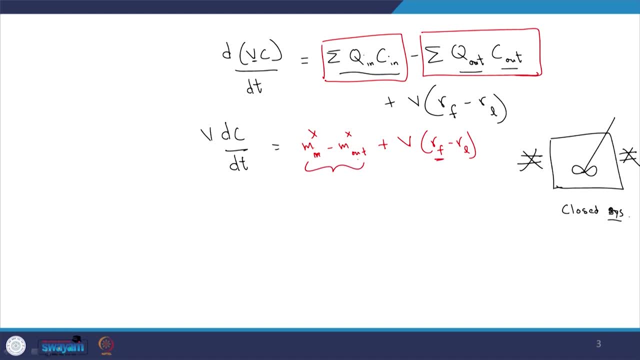 no mass leaving the system. So that is something we already looked at out here And the compound is not being formed, it is only being lost. let us say compound A is reacting with oxygen and is going to some other byproducts. let us see: 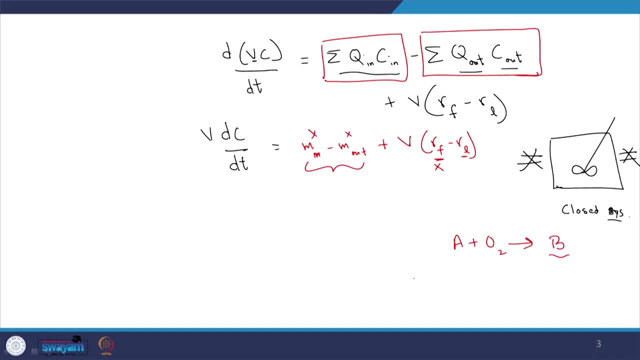 So how do I get the rate of this particular reaction here? So rate of loss? So rate of loss is equal to the rate constant of this reaction, K times the concentration of the reactants always, which are this right. So that is what we have out here. 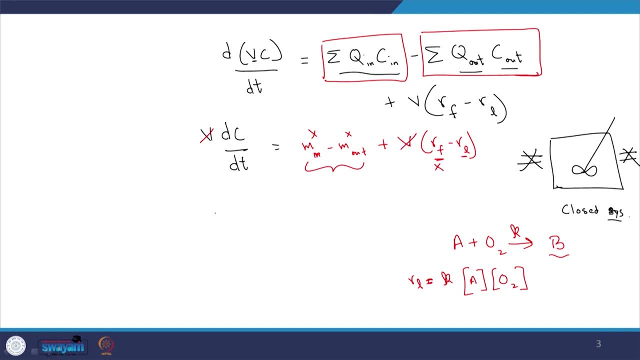 So V dC by dT, canceling out this V and V dC by dT is equal to: rate of formation is 0,. the A is not being formed here is equal to minus rate constant of this reaction. Let us say: 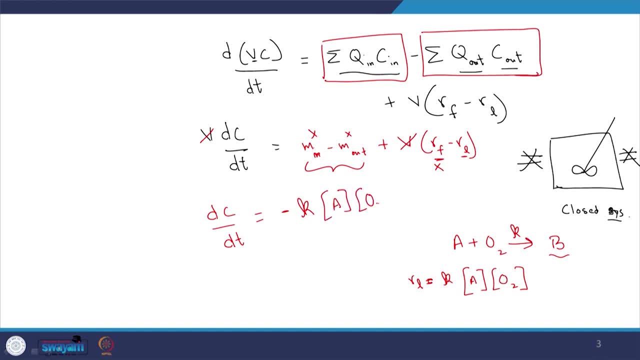 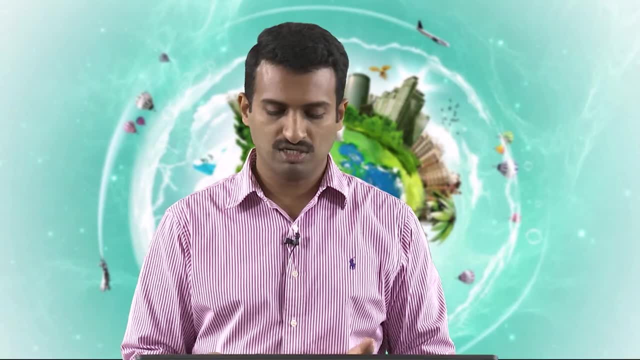 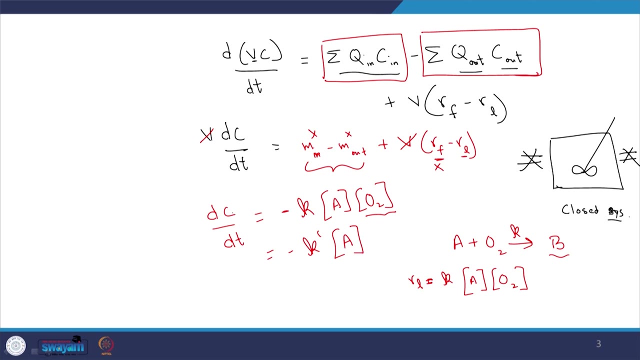 times A, times O2.. And if I know the concentration of O2 in this particular room and if I assume that it is more or less constant, I can say that it is equal to minus k, dash concentration of A. So this is C, so this C itself is concentration of A. so I can write it as: 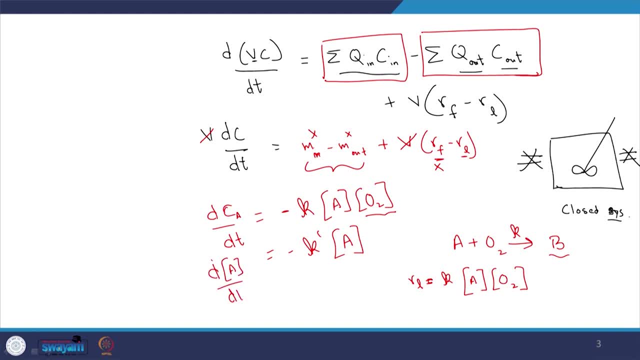 d. so these square brackets we typically use to indicate the concentration of that particular compound. So that is what I have. So this is my equation. if I integrate it, I can then understand. let me integrate it. concentration of A at any particular time- t. 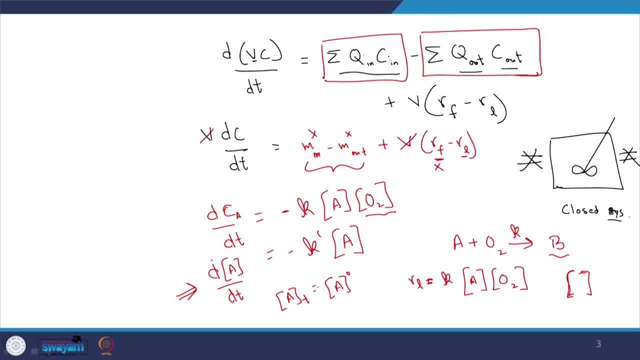 is equal, is going to be equal to A naught initial concentration, k dash t, And I want to know when this particular concentration of A at time t is going to be below a particular value. And if I know the initial concentration then I can get the time because the rate constant. 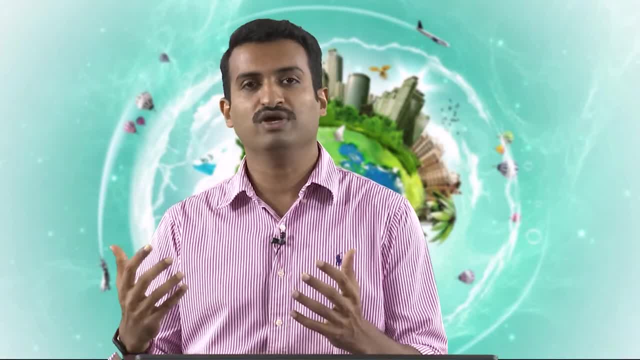 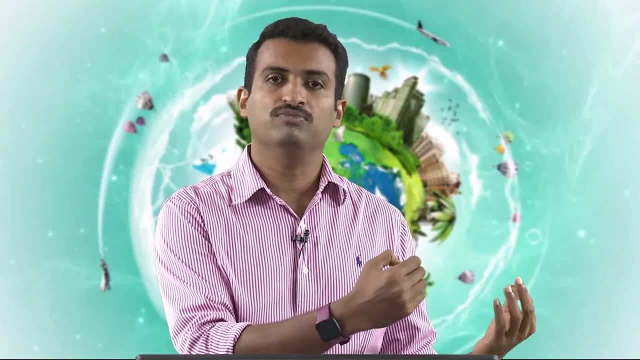 as I mentioned, is constant. So that is one way to go about it, not one way. We applied the particular mass balance to our particular system of interest and calculated the variable that we needed, which was time in this case, And this kind of closure system. 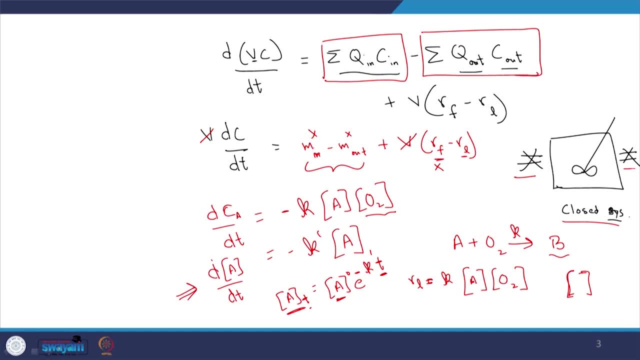 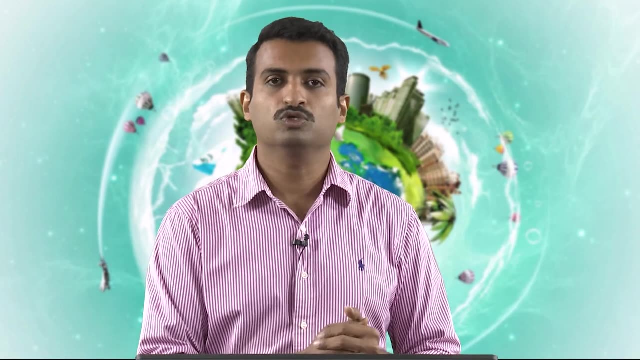 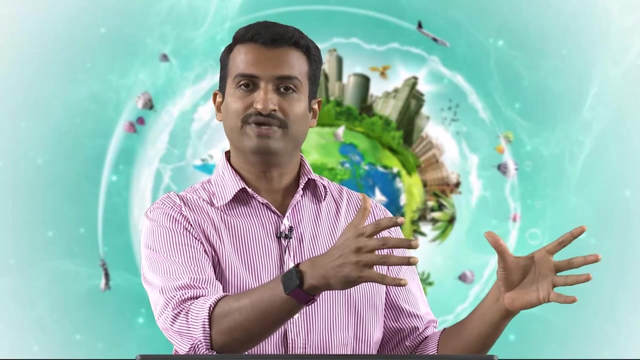 which I just described as a no mass combination and no mass going out, but which is continuously stirred, is called a batch reactor. Why do I mention this? Because you do not have the time to go through such steps. You can look at a particular reactor or a control volume out there in the field. 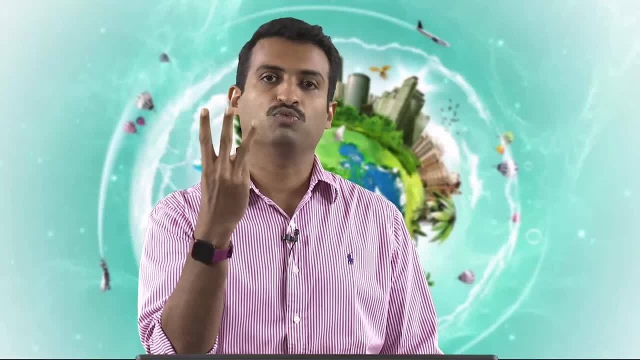 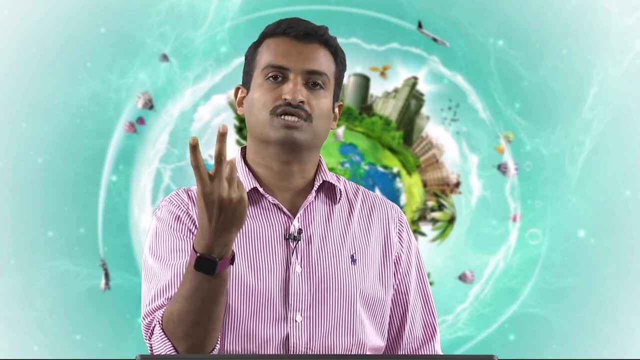 and more or less try to classify it as one of three ideal reactors: The first one we just discussed, batch reactor. The second one will be plug flow or continuously stirred tank reactor, and then the plug flow reactor, And then you will be able to quickly understand how the system is going to. 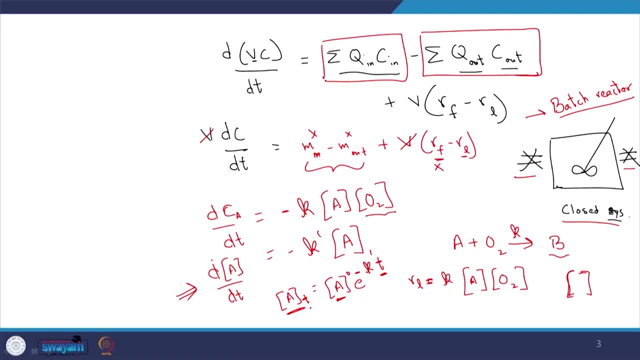 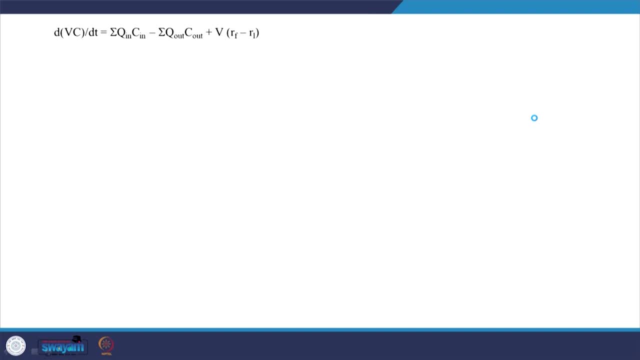 behave. So the first ideal case reactor we looked at was, or is, batch reactor. Let us move on and see what else I have out here. So this is the mass balance equation that we you will be using throughout your particular class. Please note that this is nothing but a variation of the 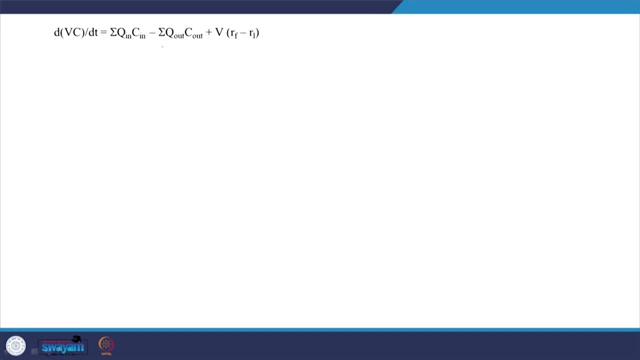 fundamental mass balance equation that we already discussed in the previous session. So what are the different variables out here, Just to be sure we are going to discuss them. V is the control volume of the system. For example, if this is my reactor in the wastewater. 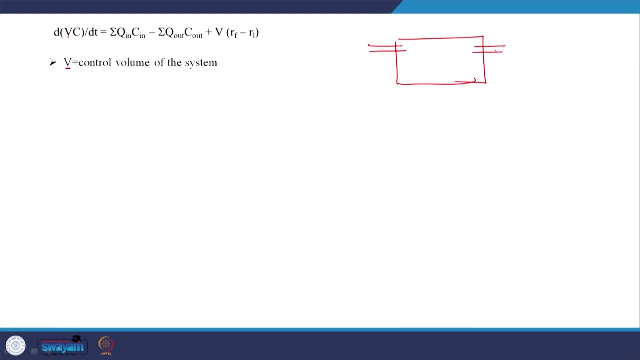 treatment plant and flow is coming in and flow is going out and this is the volume of the reactor of interest. And what next? C is the concentration of the compound in the system that I am concerned about. That C is the concentration of the compound inside the reactor. I am talking about the concentration. 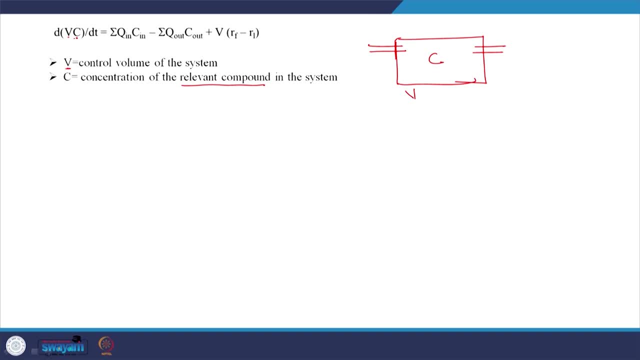 of the compound inside the reactor. this C And Q in and Q out. flow rate of the fluid coming in. flow rate of the fluid going out of the system. And C in and C out. concentration of the compound in the flow coming into the system. C in influent. 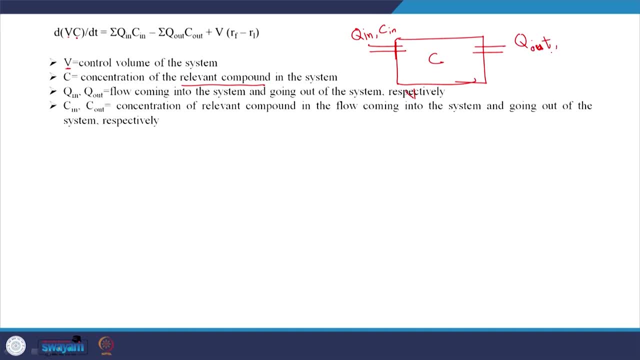 This should have been out OUT throughout, and then C out. is the concentration of the compound in the flow going out of the system C out? And what else do we have? rate, RF, rate of formation of the compound in the system and rate of loss of compound in the system. 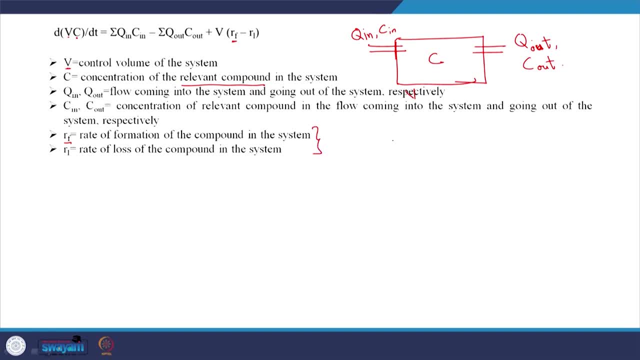 And just to refresh your memories with respect to the what is it now? chemistry here. So let us say I have A plus B goes to C plus D. The rate of the reaction is equal to the rate constant. rate constant which is depend upon temperature and pressure, but typically 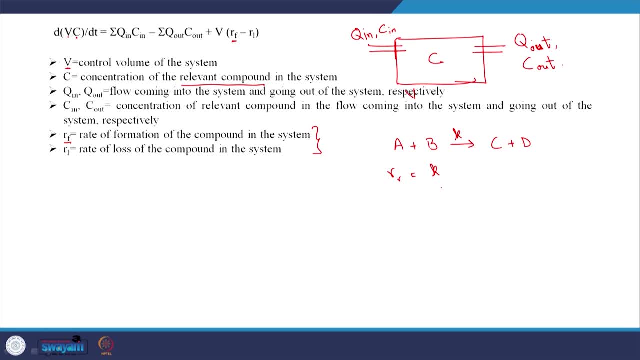 temperature is what we are concerned about, assuming the pressure is relatively constant- into the product of the concentrations of the reactants. It depends only on the reactants. Keep that in mind- rise to their stoichiometric coefficients. Here there are no stoichiometric coefficients. 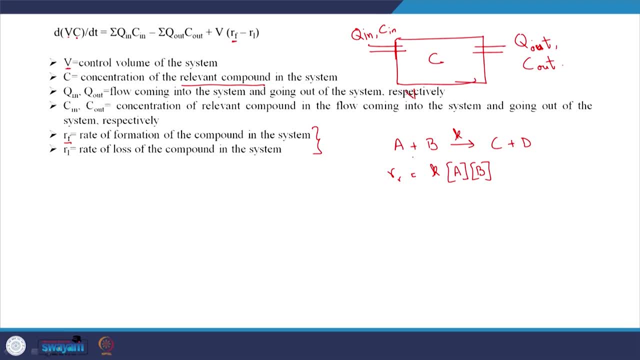 That is something to keep in mind. But if I transform it such that I have, let us say, these are the stoichiometric coefficients, And then what is this rate equation going to be like? K times A rise to its stoichiometric coefficient, and concentration of B rise to its stoichiometric coefficient. 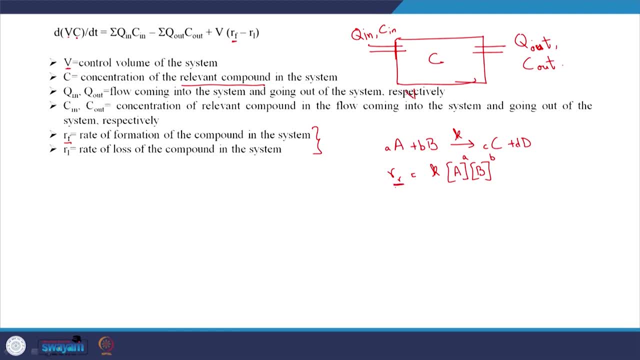 As I mentioned, this is the rate of the reaction. but how do we relate rate of the reaction to the individual Rates of the formation or loss of the compounds? here, For example, rate of reaction is what I have and I want to be able to get that to rate. 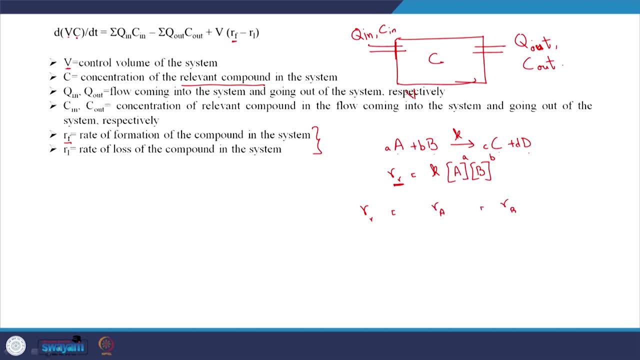 of A rate of loss or increase or formation of B or C or D. How do I do that? So that is, by using the stoichiometric coefficients. So that is going to be equal to by A and negative, because A is being lost by B negative and 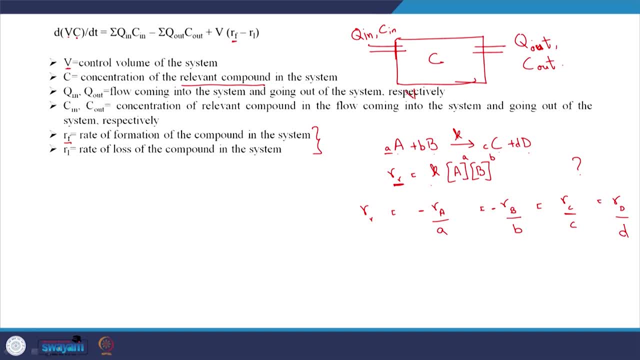 C and D. So that is going to be equal to by A and negative, because A is being lost by B negative and C and D. So, for example, the rate of loss of A- because I am specifying it as loss, I can remove the. 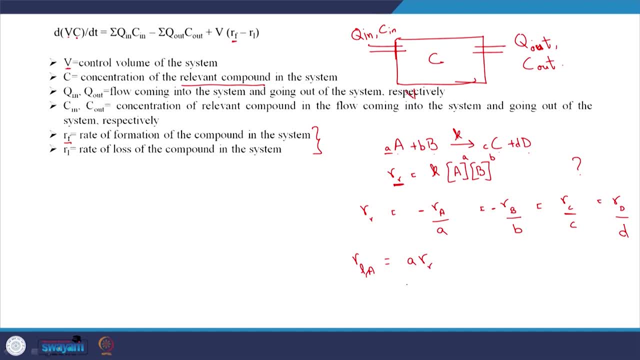 minus term here is going to be equal to A into rate of the reaction. So that is equal to A into what is the rate of reaction? we have that out here: K times: concentration of A: rise to its stoichiometric coefficient. concentration of B- rise to its. 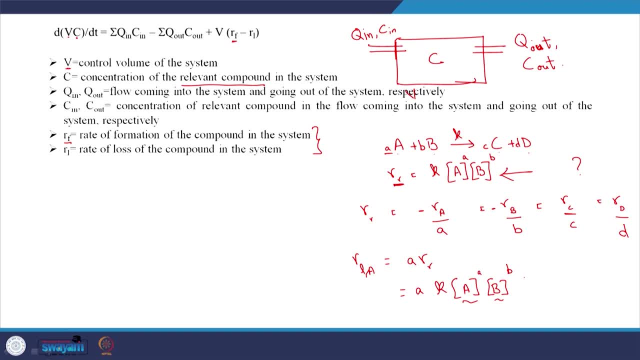 stoichiometric coefficient. Why A and B? Obviously because the rate of the reaction. Why A and B? Because the reaction only depends upon the reactants and not that of the products. For example, RC rate of formation of C is equal to C. the stoichiometric coefficient? 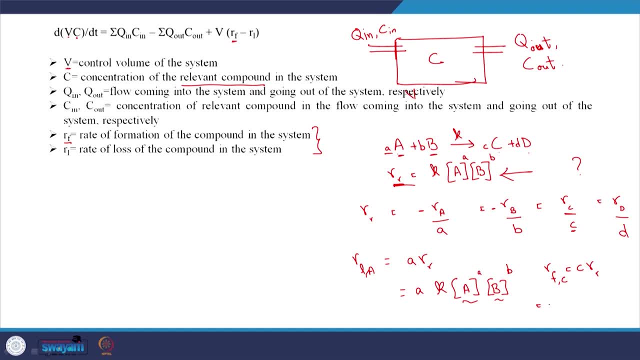 of C times the rate of the reaction- So that is equal to C times K- into concentration of A: rise to stoichiometric coefficient of A. concentration of B: rise to the stoichiometric coefficient of B. So you have to be careful about this negative term. 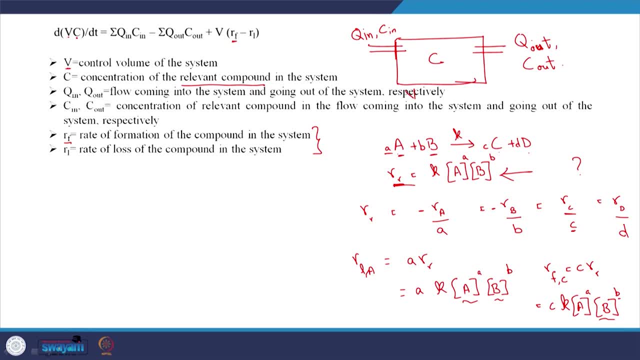 For example, when I wrote in the mass bands equation term here rate of formation minus rate of loss. you should not see to it that you write rate of loss as minus of you know some particular equation and you have two minuses out here and they cancel out and become. 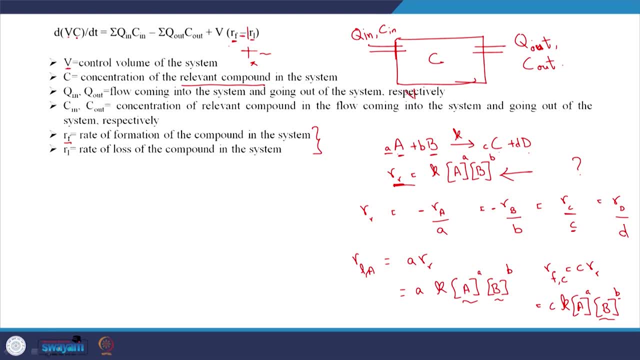 a plus. That is not what you have Here. we are writing minus, assuming that not assuming because it is rate of loss. So you should not have another negative symbol for the rate of loss. Okay, plus out here, right? So that is something that you have to keep in mind out here. 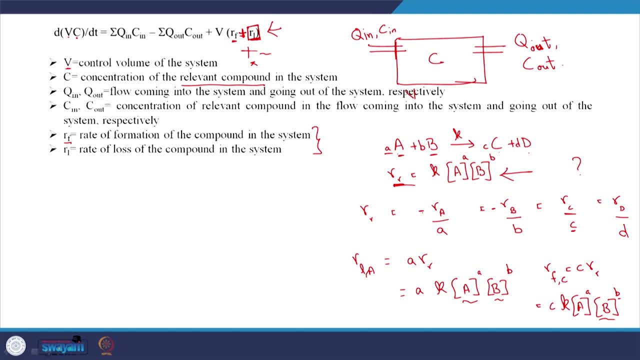 That is why here I did not write rate of loss or such. that is why I wrote the negative term here, as in: A is being lost, A and B are being lost out here, while C and D are being formed. that is why positive out here and negative out here. But because I wrote rate of loss here I did not use 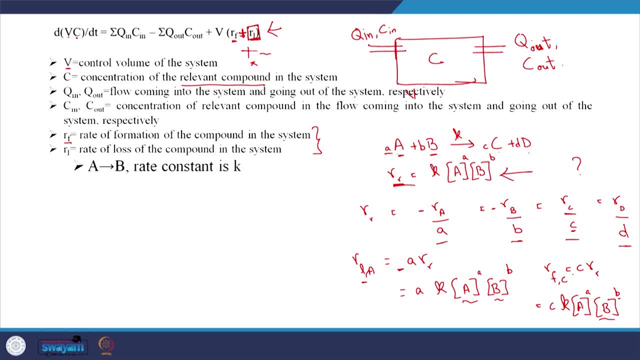 any particular symbol out here. that is something to keep in mind. So what do we have? I guess we have more or less a review of what we just discussed. A goes to B. rate constant is K. rate of the reaction is K times rate constant: K times the concentration of the reactants, which is 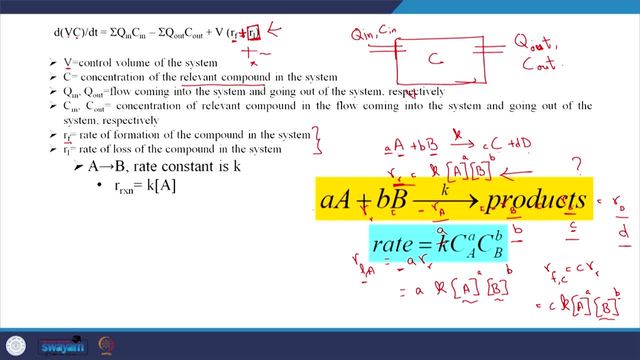 A right And I guess, if it is this particular relationship out here we are going to have: rate of formation of A is 0 and rate of loss of A is equal to rate of reaction times- the stoichiometric coefficient- That is something that was missing, obviously- and rate of formation of B. 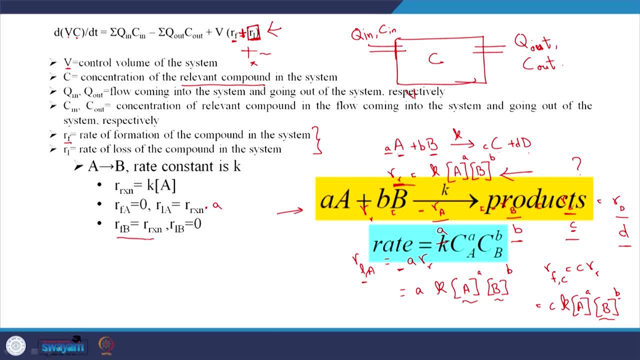 is rate of formation of B. well, I guess obviously this is not the equation for this particular term. okay, I understand what I was trying to do. This set of information is for this reaction out here and not for this one. So rate of the reaction. this reaction is K times concentration of A and as we 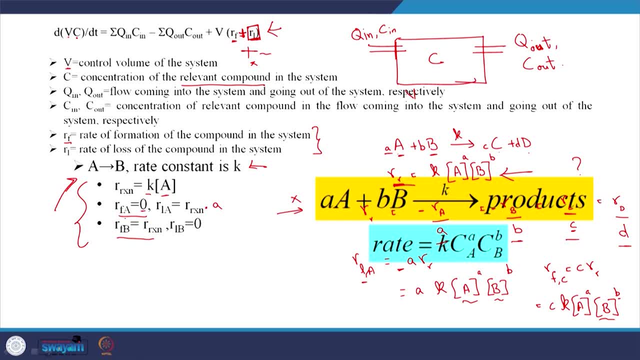 see rate of formation of A. A is not being formed. that is why it is 0.. Rate of loss: loss of A is equal to the rate of reaction of A times stoichiometric coefficient of A, which is 1.. And rate of formation of B, as you see, is going to be equal to 1 times the rate of the reaction. 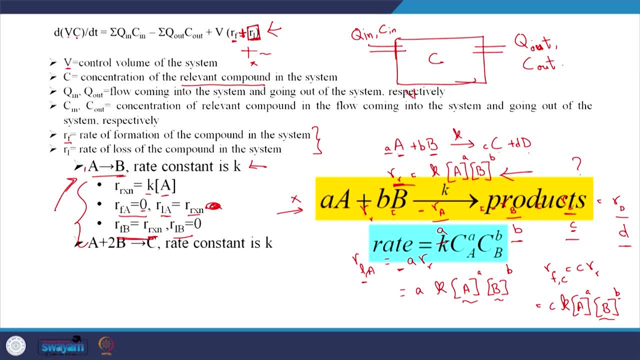 rate of loss of B is equal to 0 out here. right. But if it is A plus 2, B goes to C and rate constant is K. what do we have? Rate of the reaction is K, rate constant times concentration of A into B to the power of stoichiometric coefficient, which is 2 out here. 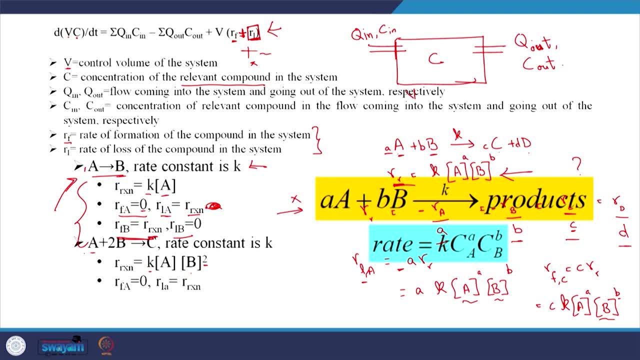 And rate of formation of A is 0. because A is only being lost and rate of loss of A is equal to 1 times the rate of the reaction. why 1? because the stoichiometric coefficient of A here is stoichiometric coefficient of A, here is 1 right. 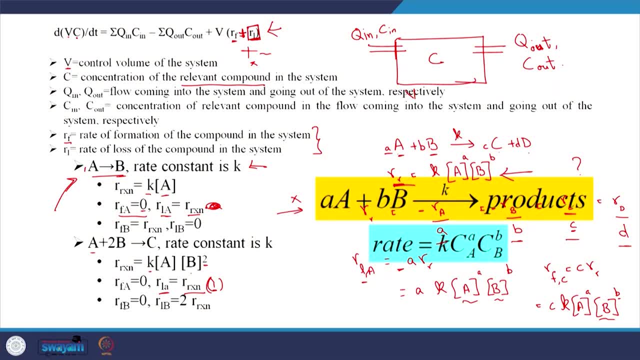 So that is something to keep in mind. and similarly, rate of formation of B is 0 and rate of loss of B is the stoichiometric coefficient of B, which is 2 times rate of the reaction. And then rate of formation of C is equal to the stoichiometric coefficient of C, which is 1. 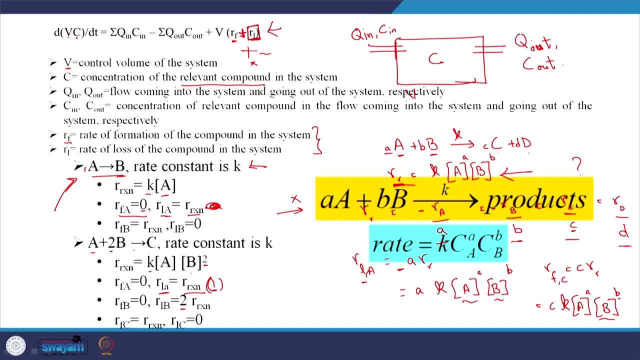 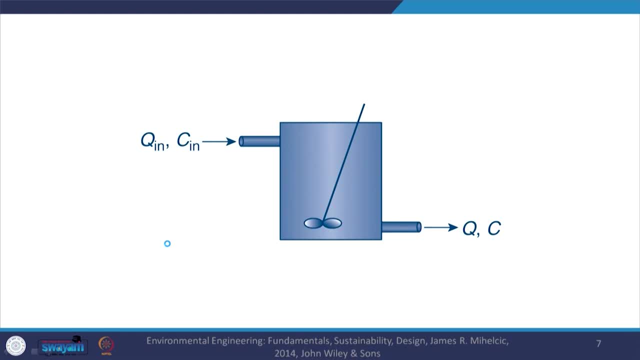 times rate of reaction and rate of loss of C is equal to 0 because, as you see, C is only being formed, it is not being lost. So that is something that we have out here, And we looked at the case of batch reactor earlier, as in, this is my reactor and no flow is coming in and no flow is going out. 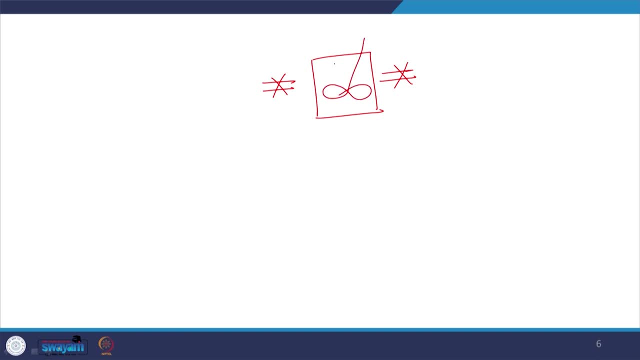 while assuming that it is completely mixed, meaning the concentration of the compound within this particular rate of formation of C is equal to the stoichiometric coefficient of C. So for that V dc by dt is equal to mass coming in Q n, C n minus Q out, C out plus volume into rate of. 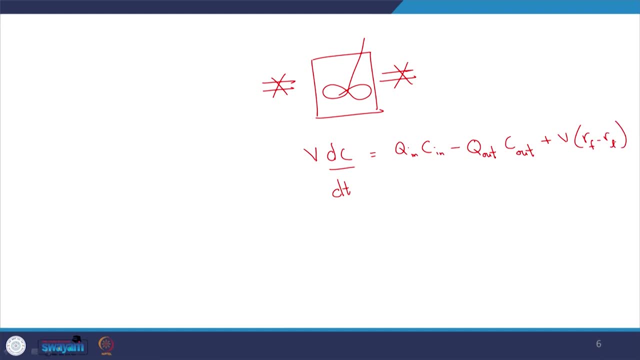 formation minus rate of loss. So this is the mass balance equation that we are going to use throughout. So summation term here, but assuming that there is only one flow. So these terms turn out to be 0 for the batch reactor right: Ba t Ch batch reactor. 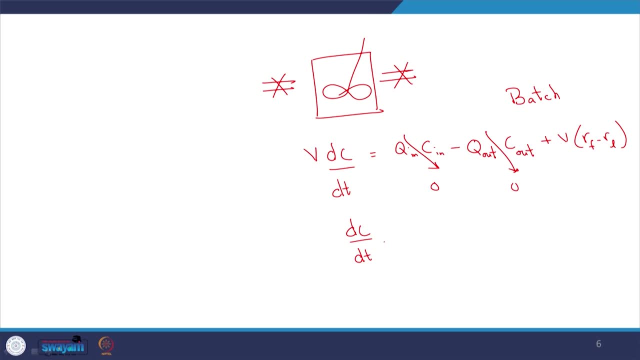 And just ends up being dc by dt is equal to rate of formation of the compound minus rate of loss of the compound. If you have that information you can solve that. So next kind of system is modification of the batch reactor as an. we still have continuous mixing. 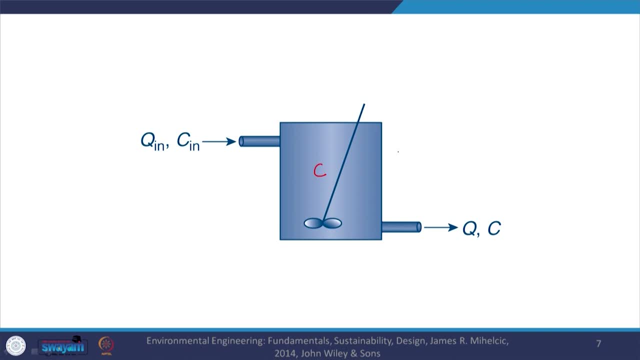 so the concentration of the compound inside the reactor is the same throughout the system system. But unlike the earlier case, we are going to have mass coming in and mass going out. let us see- and this is from this reference particular book out here- Environmental engineering fundamentals, sustainability, design and design. 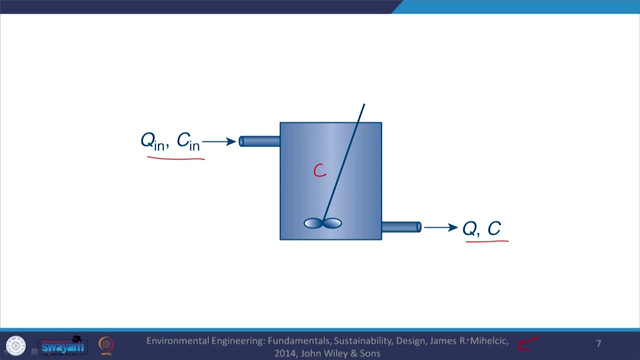 Note that you know this is a generic figure and can be taken from anywhere, or we can draw that too right, But I wanted to mention that reference because that is one of the other. what do we see? supplementary references you can always look at. So we have this particular information. let us try to apply the mass balance equation. 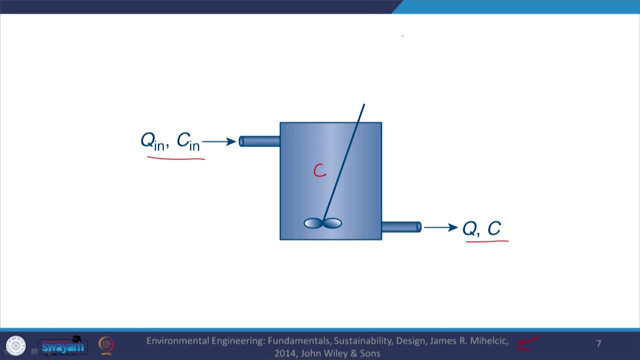 to this When I say this. how do I describe this kind of a system? So it is either called a continuously stirred tank reactor or continuous, continuously stirred. right, it is always stirred tank reactor. So it is called CSTR, or another name is CMFR, as in completely mixed flow reactor. 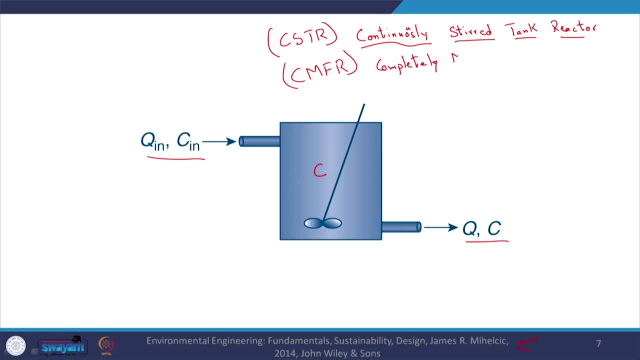 So basically it is a mixed flow reactor. Okay, So both these terms are used to describe this system. So the system is that we have mass coming in and mass going out, or flow coming in and flow going out, and the compound thus flowing into the system and going out of the system. 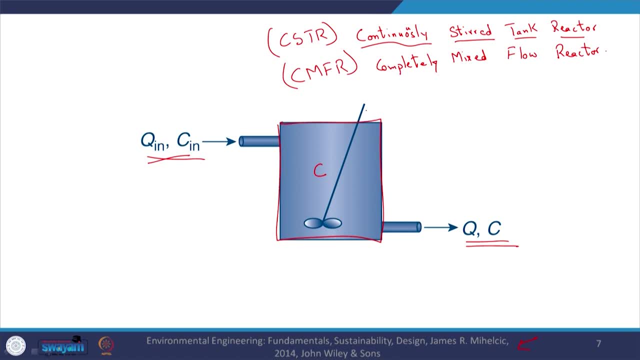 What is my system? This is the control volume, and it is continuously stirred or completely mixed, always. So that is something to keep in mind. Now let us try to apply the mass balance equation to this particular system out here. So we have V dc by dt. 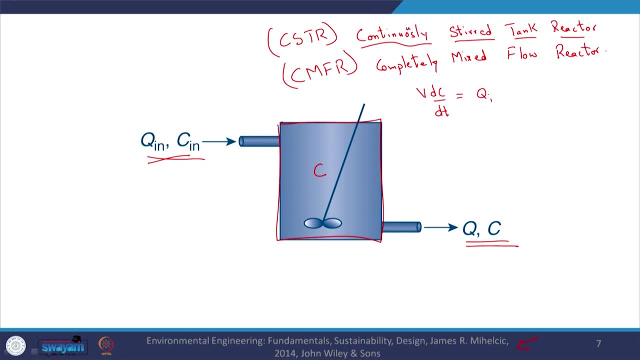 Is equal to Yes, Is equal to Q in, C in minus Q out, C out plus volume, into rate of formation minus rate of loss. Let us say we are assuming steady state for the sake of simplicity, but we can always. if the system is not at steady state, then obviously this term would not be 0.. 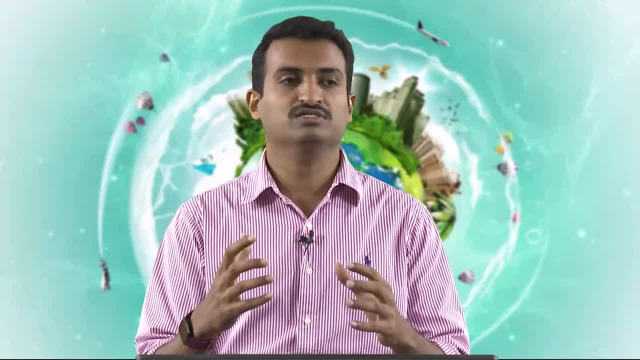 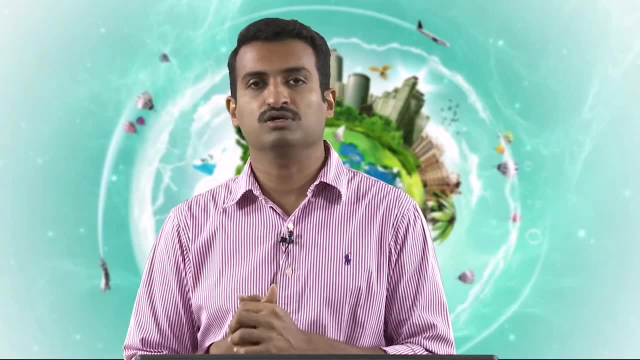 So what do I understand when I say that system is steady state? it means that if the system is at steady state, all the variables- please note that it is every variable, not just concentration or such- all the variables are constant with time. there is no change in any variable in. 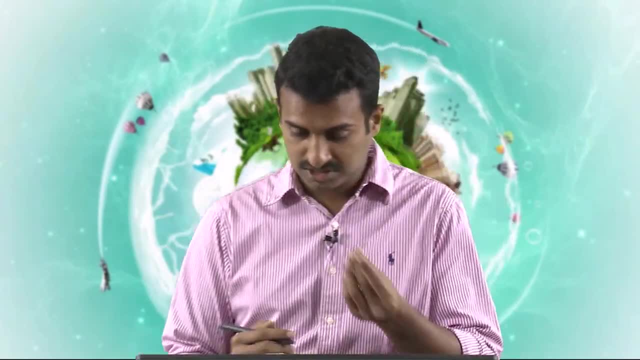 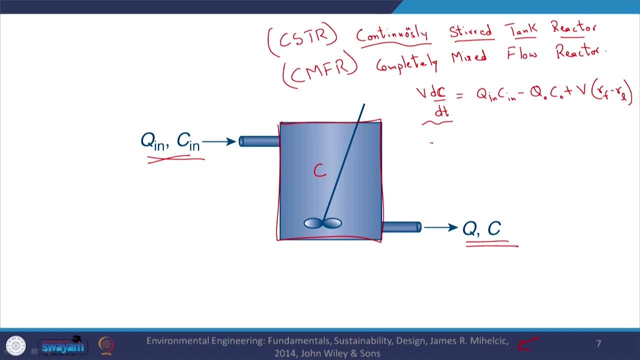 that system with time. So obviously, if the system is at steady state, that obviously means concentration too does not change with time. So dc by dt is going to be 0, assuming that it is at steady state. at steady state, Let me write it down for the first time. 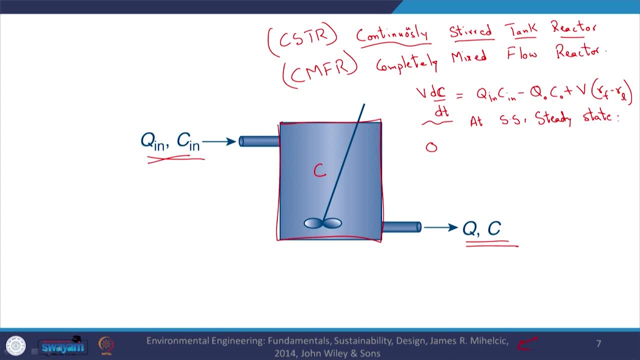 Steady it is. steady state is equal to Q in C in Q in C in minus. and one aspect to notice, because if the concentration of this particular- not concentration, pardon me- volume of this particular reactor is the same, and the fluid volume too does not change with time, 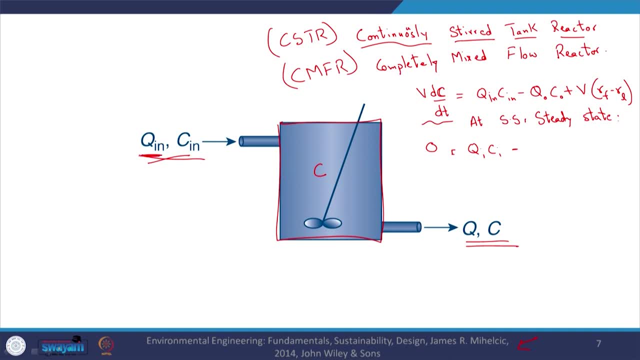 let us say then: that has to be the case, or that will be the case only when Q in and Q out are the same. So rather than writing Q in and so on, from now I will just use the term Q. the flow coming in will be equal to the flow going out. 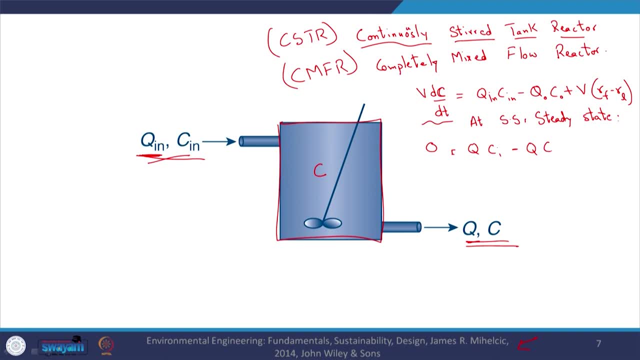 And concentration coming in minus Q into Q, Okay. Concentration going out plus volume into rate of formation, minus rate of loss. Let us just try to simplify this a bit more or further. But to simplify this further, let us say: if I have no formation but loss, for example, 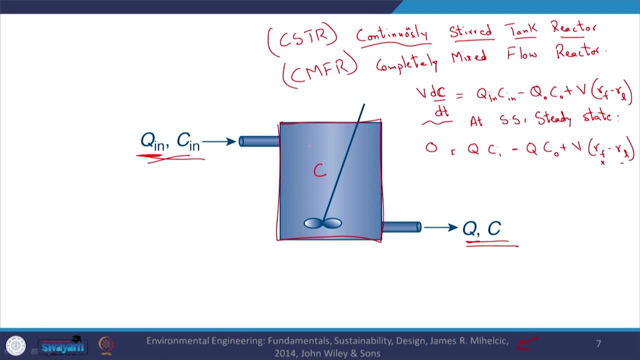 assume that the compound of interest is being lost by a first order reaction. let us say A is my compound of interest and it is going to product Okay, And the rate constant is K. it is not being formed and that is the reaction of concern. 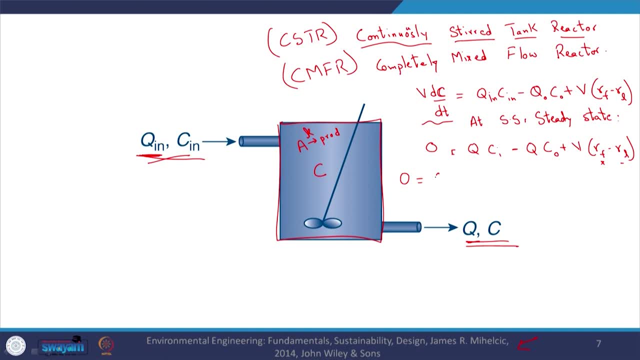 here. So what is it going to be? U is equal to Q times C. coming in minus C. going out plus volume into, there is no formation of the compound, as we just saw, 0 minus. how is the compound being lost by this reaction? 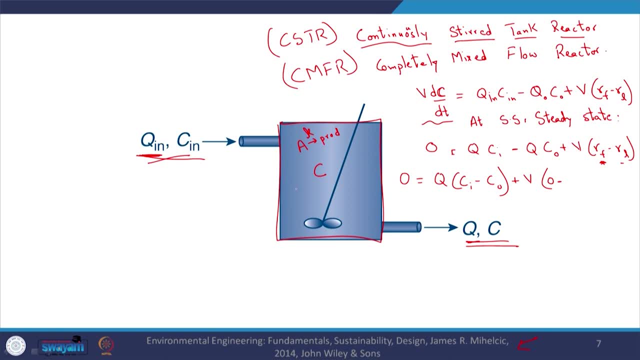 And what is the rate of loss of this particular compound? A, That is, the rate of loss of A, is equal to the stoichiometric coefficient 1 times rate of the reaction. And what is the rate of reaction? It is nothing but K times concentration of A within the reactor. 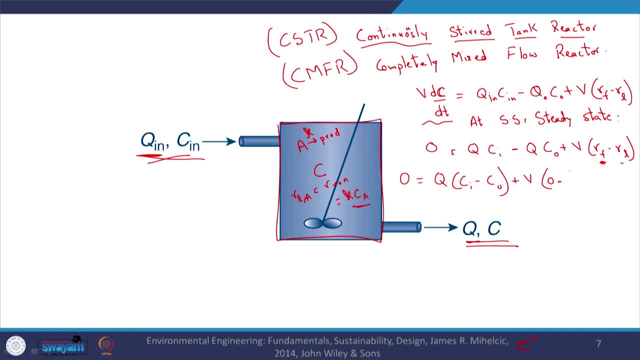 Right. So that is what I have and that is what I am going to plug in here- is equal to minus concentration of A within the reactor when I say A concentration of A in the reactor. But here I know the input. Okay, Right. 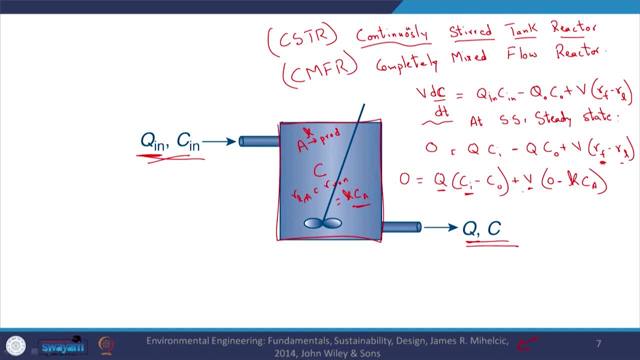 I know the flow volume of the system. I will know because it is a rate constant, I will can get the rate constant. But the issue here is I have only one equation but I have two unknowns as in concentration going out of the system and also concentration of the compound within the system. 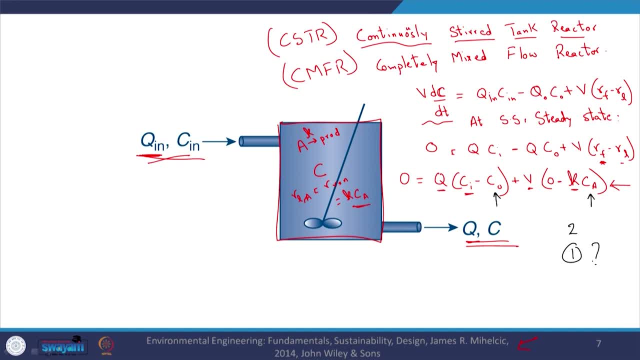 So I have two unknowns but only one equation. So how do I solve this? The issue here is that if you observe the system, or if you understand the system, it gets continuously stirred or completely mixed. So the concentration of the compound here within the system is always the same at all. 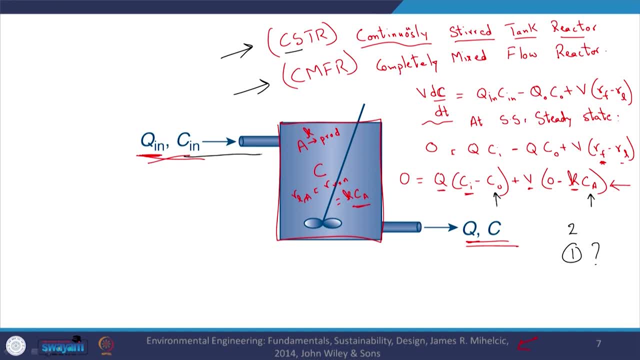 locations Right. And what does that mean? The constant: once the compound comes in, it is immediately diluted to particular concentration, CA. And if the concentration is the same throughout the reactor, what does that mean? That means that the concentration of the compound going out of the reactor is also going to. 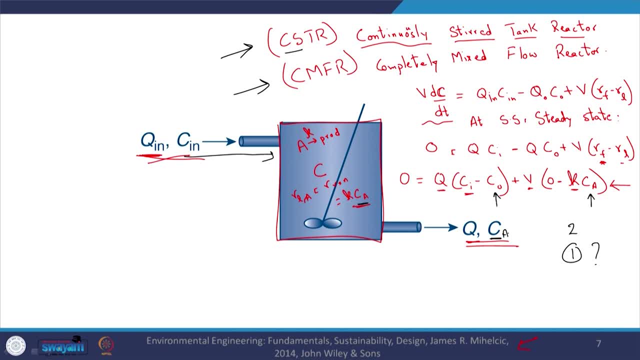 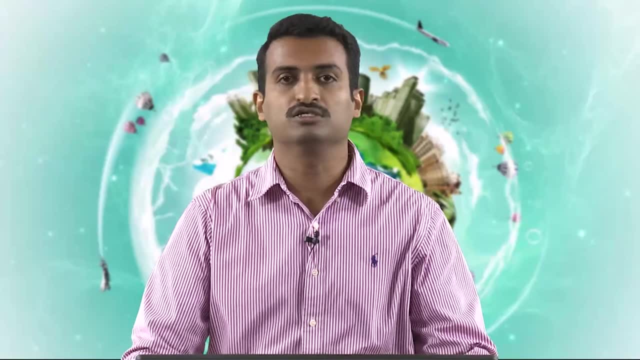 be equal to the concentration of the compound, The compound inside the reactor Right. Why is that? Because if it is completely mixed and the flow is going from the reactor outside the to outside the reactor, So the concentration of the compound leaving the reactor will be the same as the concentration. 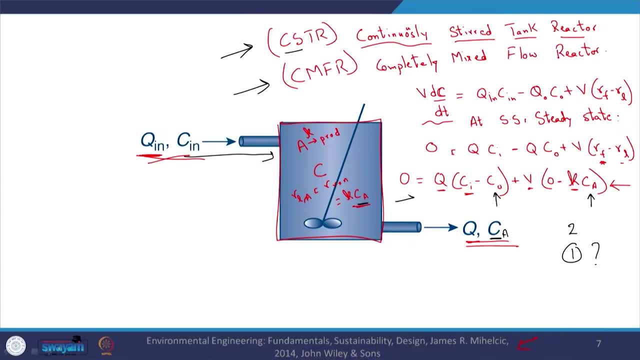 of the compound within the reactor. So with that information, what can I do? 0 is equal to Q into C in minus C out. I will just say C Plus Right Volume into minus K. concentration of compound inside the reactor. I will just say or refer: 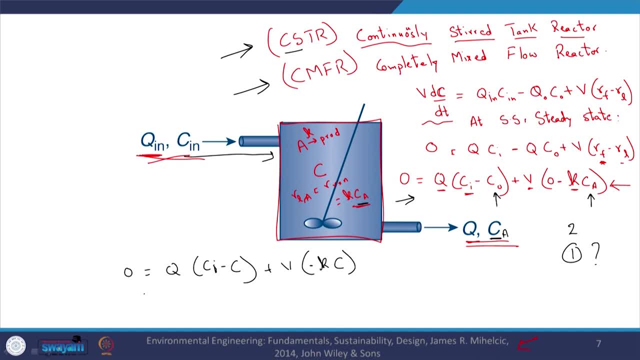 to it as C. Right Now, if I play around with these variables to be able to or try to solve for C, Let us see what I will have. I will try to take this term, this term and this term to the left hand side. 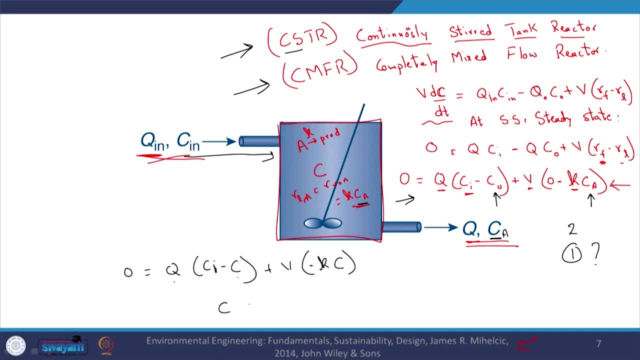 So what will I have out here? I will have- let us say, I will take C as a common term. out here I will have: Q Right Plus volume into K is equal to Q into C. i Right, And hopefully I did not commit any silly errors. 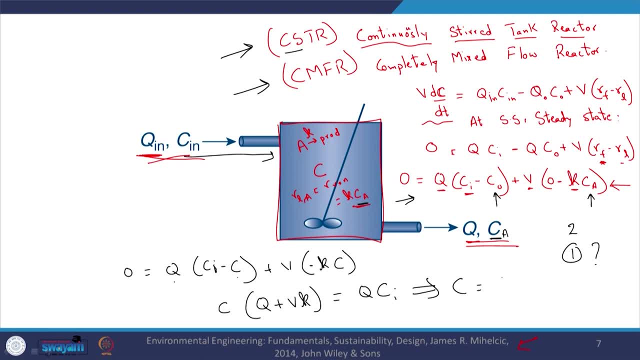 So concentration of the compound leaving the system is equal to Q into C, i by Q plus volume into the rate constant. This is when, obviously, we have a first order loss. Obviously, This is not the case. It is going to be different Again. keep in mind that. how did we end up at this? what do we say? equation. 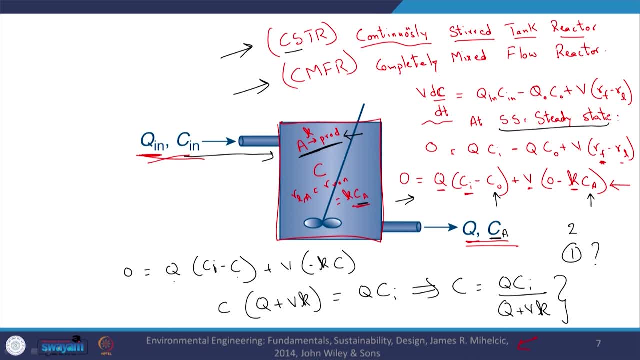 We assume that, first, that the system is at steady state, We assume that the compound is not being formed. We assume that the compound is being lost via a first order loss. With that we ended up with this particular equation. So again, continuously stirred tank reactor, and this is something that we are going to. 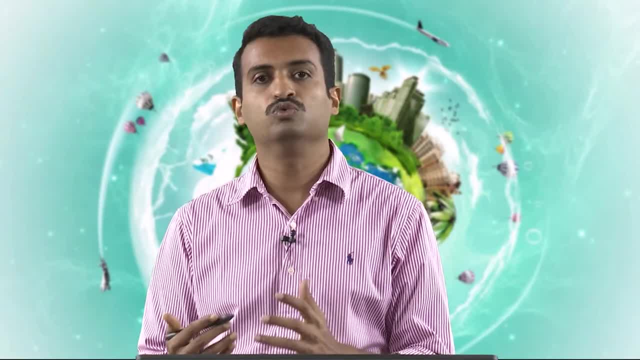 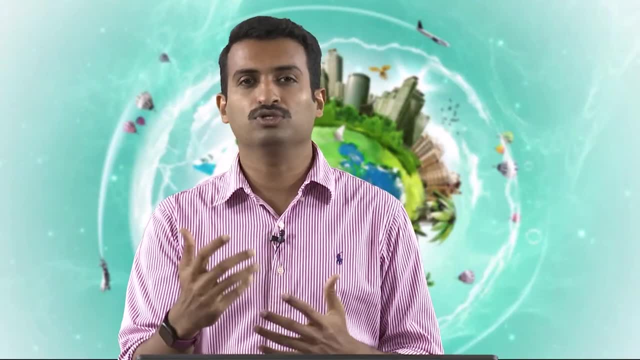 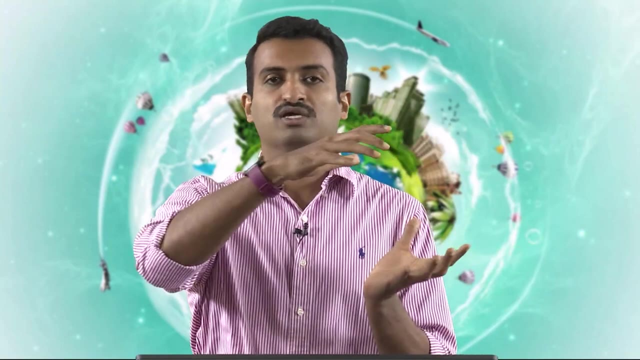 use throughout the class. That is for you to keep in mind. Why is that? you know, if you look at general wastewater treatment plants, which I am going to call by activated sludge process for now, we will understand what it is later. So you are going to have our wastewater flowing in to this particular activated sludge tank. 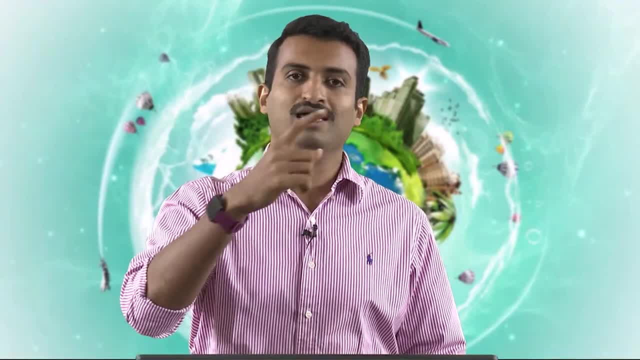 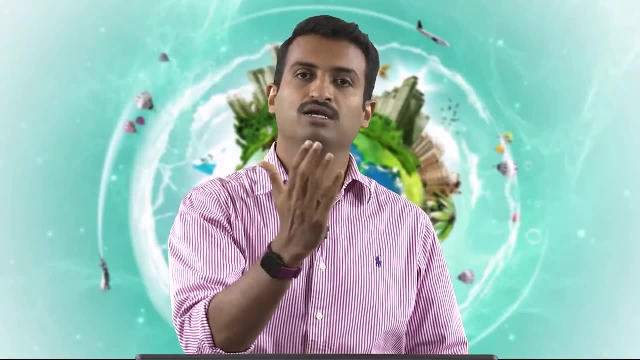 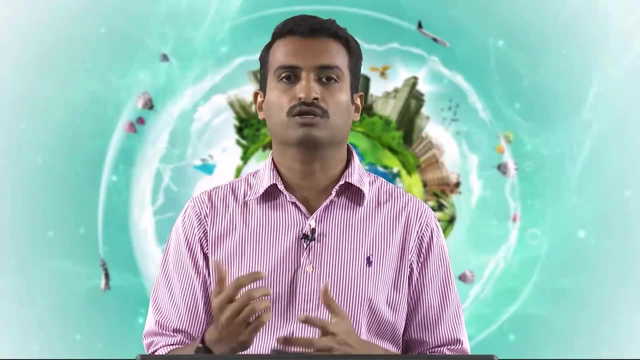 and wastewater always flowing out And we are going to provide air for the oxygen, for the microbes, So you are always also going to provide oxygen Right. This will lead to mixing and more or less same concentration throughout the reactor. So more or less that is a continuously stirred tank reactor or completely mixed flow reactor. 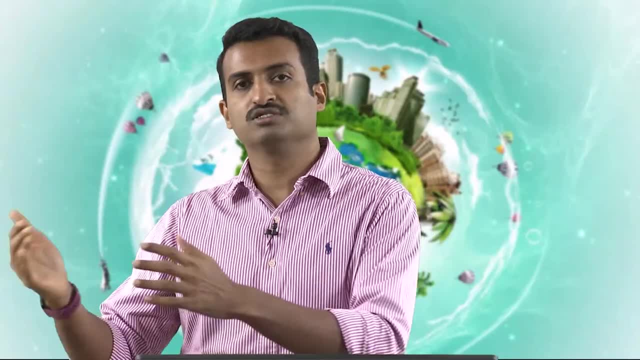 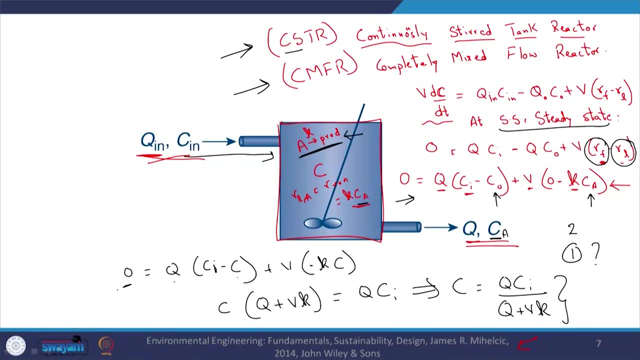 Please note that it will not always be an ideal reactor, but we will discuss this in the next session, I guess. Again, let me just wrap it up. So what did we have? We have steady state out here: Mass coming in, mass going out and the reaction or the mass being lost by the particular reaction. 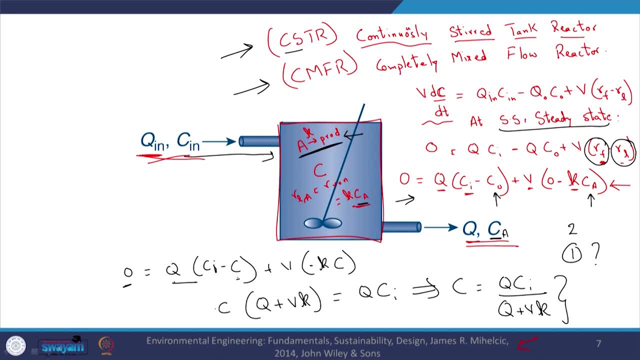 out here. So taking these terms out to the left hand side and taking C out as the common term. So Q minus, C comes out here plus, So I take C- it is Q and VK is equal to Q into CN and end up with this particular system. 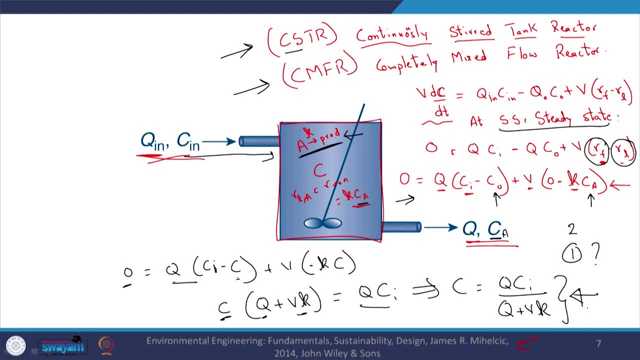 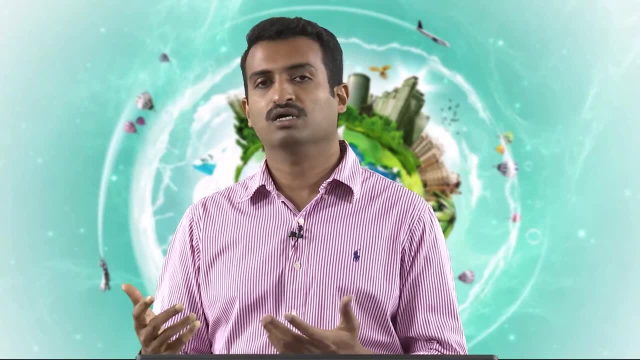 Typically mugging it up is not a good idea in this class at least. whenever I am going to give the, whenever you are going to take the exam, Most of the formulae are going to be given. but if it is simple- mass balance equations and such it. 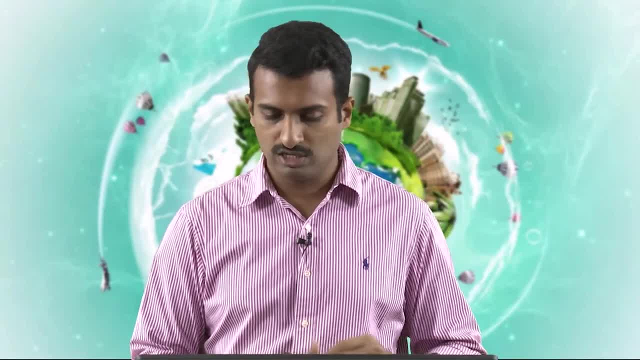 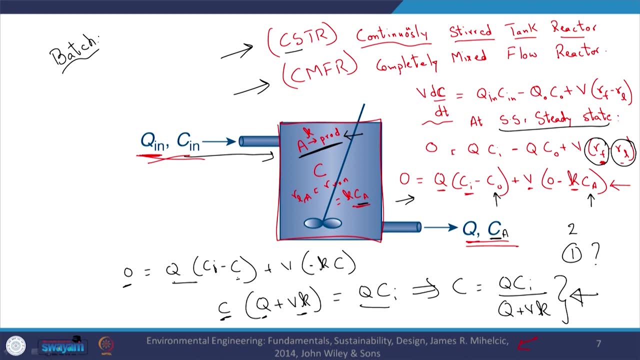 I will leave it up to you to be able to solve it. So that is something to keep in mind out here. So until now, we looked at the batch reactor and then we moved on to looking at this continuously stirred tank reactor or completely mixed flow reactor. 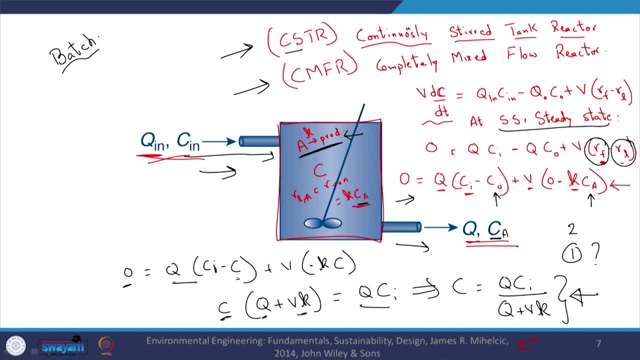 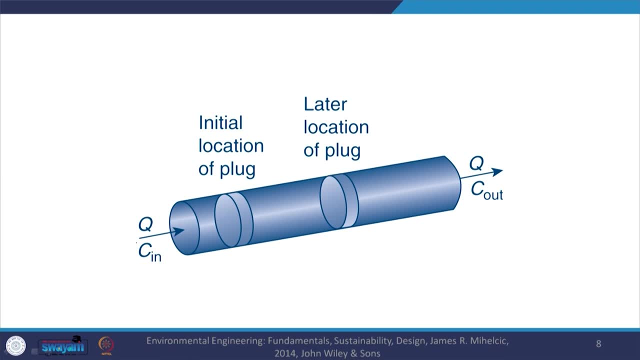 As in, unlike the batch reactor, we have mass coming in and mass going out. The next one is more or less variation. as in, we have mass coming in and mass going out, But, unlike the continuously stirred tank reactor, there is no mixing inside the reactor. 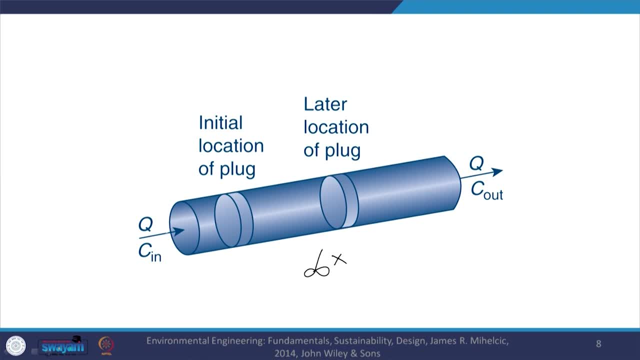 So if I, in an ideal case, plug flow reactor, if I release a tracer here after particular time and thus distance, I should not say time after particular- after the plug has travelled a certain distance, the shape is going to be like this: and even after X2 distance, after 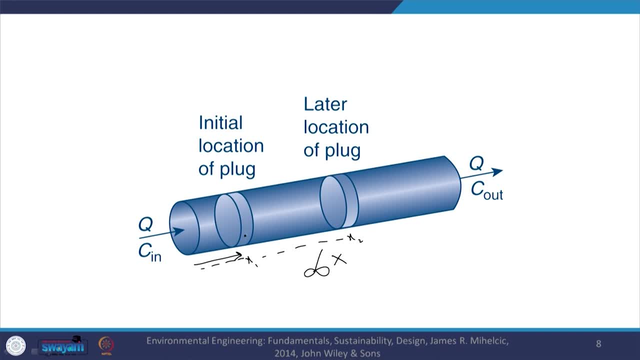 it has travelled x2.. The shape of that plug, original plug, will be like this: why is that? there is no mixing right? there is no mixing out here. That is why it is called a plug flow reactor right. that is something to keep in mind. 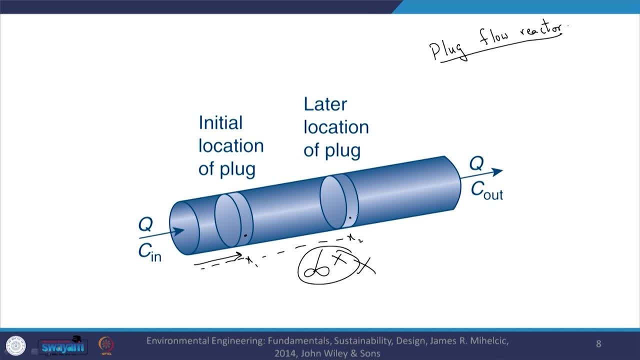 So within this control volume. so this particular cylindrical shaped reactor is my control volume. there is no mixing. So how does the concentration change? The concentration changes because as the plug travels along the length of the reactor, it undergoes reaction and it will lead to loss of your particular compound. 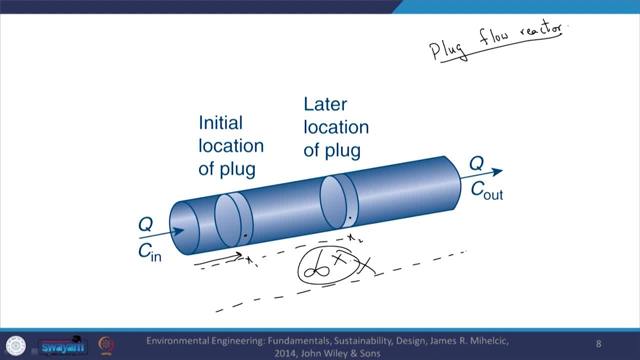 So let us just try to apply the mass balance equation here and see what is the issue. or can I directly apply the mass balance equation here? V dC by dt is equal to Q in, C in minus Q out, C out plus volume into rate of formation, minus C out. 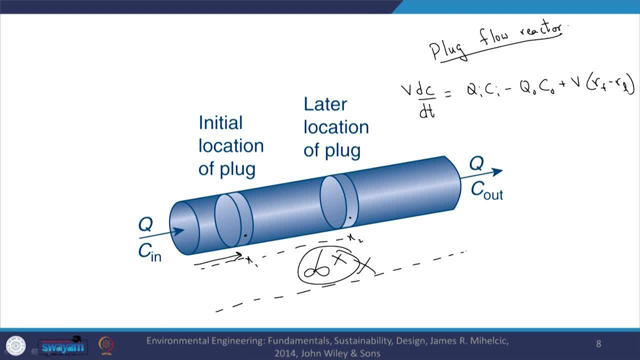 Minus rate of loss- right. But if you look at this equation here, we see that we cannot really apply this equation out here. Why is that? Because in this system for first order loss or such, you see that the concentration is changing with distance. 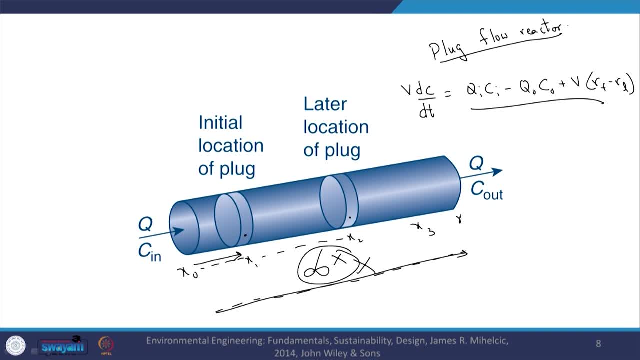 That said, this is X0, X1, X2 and X3 and X out. So concentration is changing with distance, Right. But in this system we see that there is no such flexibility, at least in this equation- pardon me, the fundamental, not fundamental- the macroscopic mass balance equation as we 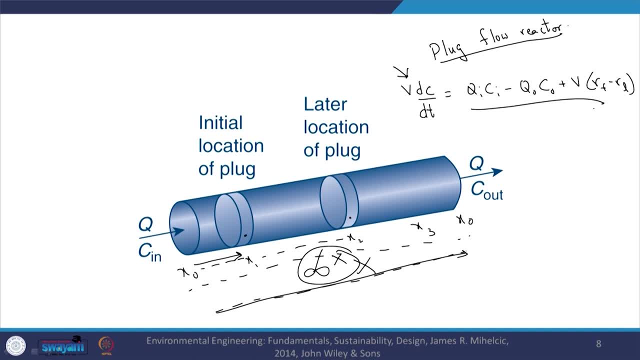 wrote down out here. we see that. you know it is more or less built in for systems within which the concentration of your compound is the same. But here for our plug flow, we see that it is changing. out here it is different out here and such. 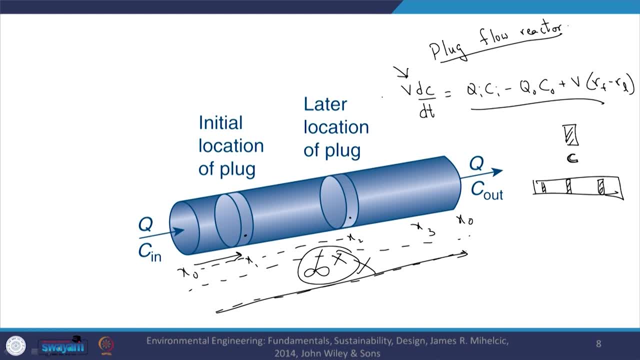 Right, The concentration of the compound is changing with distance, So I have to transform this equation so that I can apply it to my plug flow reactor. We will do that in the next class But, as I mentioned, you can always use your fundamental mass balance equation. 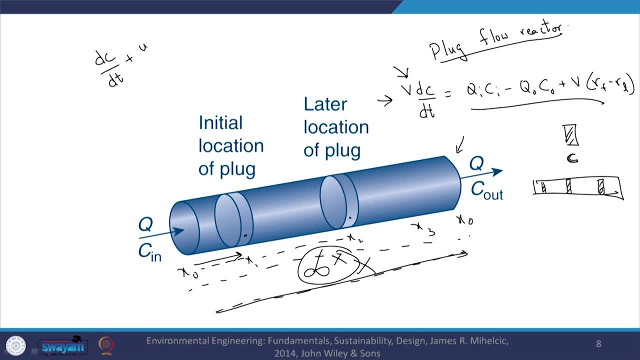 What was the fundamental mass balance equation, which can be used for every type of reactor with some transformation or the other. That is what we have. Right Is equal to rate of formation minus rate of loss. But here, as you see, You have concentration change with time, concentration change with distance and the rates of the 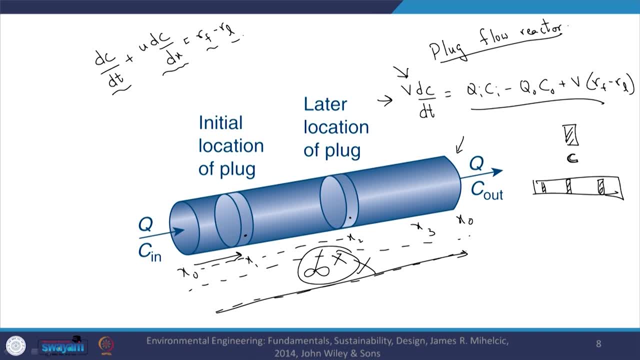 different formation and loss reactions. So if I want to apply it to this reactor or the plug flow reactor PFR, which I call as plug flow reactor- Please note that these are all ideal case reactors- What can I do? I can directly apply this particular equation. 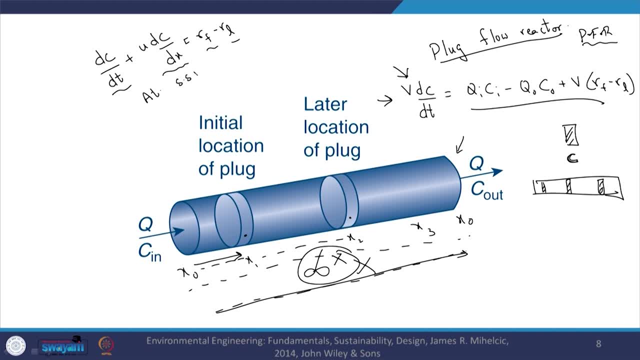 So if it is at steady state, What will it Transform into? So this particular term will be 0 and u. dc by dx is equal to rate of formation minus rate of loss. Right, But if I look at transforming this further, what is x by u? 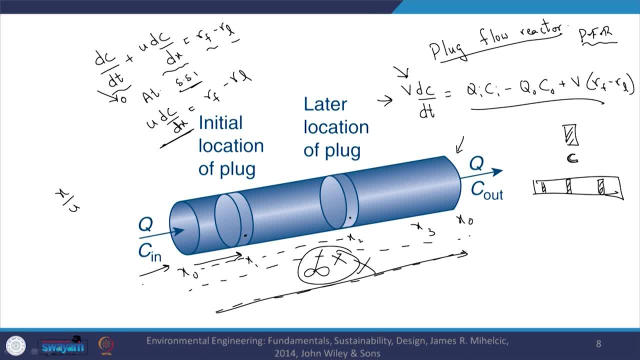 x is this distance and u is the velocity of flow of this fluid. So what will x by u give me an idea about? it will give me an idea about the time. let us say If it is x1.. Okay, And what does that mean? It spends a time of it, meaning the compound or the fluid spends. 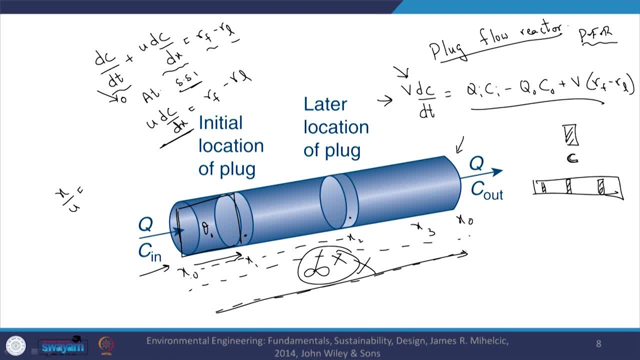 a time of theta 1 inside that reactor, or it takes a time of theta 1 to travel a distance of x1.. So x by u. I am going to call it as theta or the hydraulic retention time. I will write that out here: Hydraulic retention time. It gives me an idea about how much time the 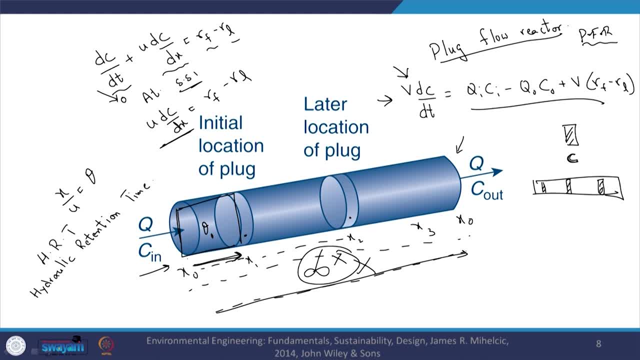 particular compound or by conjunction, the fluid. how much time the fluid or the compound spends in that reactor x by u? People sometimes think that it is the time that is changing here it is not. Keep in mind that the concentration is 0. It is not changing with time because we already assumed that it is at steady state, The concentration. 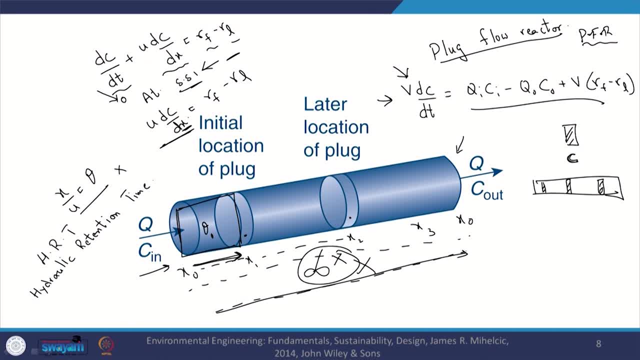 is changing with distance. That is what we see out here, So that is something to always keep in mind. the concentration at steady state is not changing with time, but it is changing with distance. We are only transforming it by writing x, which is a variable, and u, which